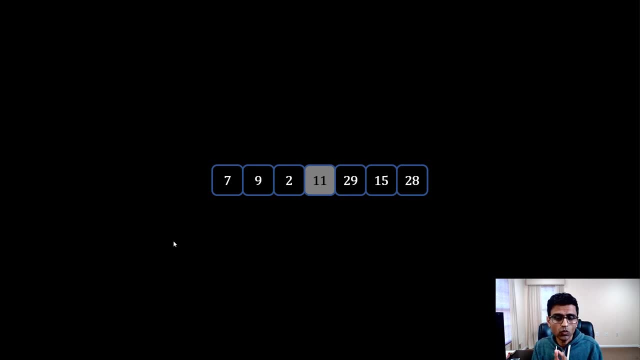 this element is sorted. Now we focus on left hand side of an array. So we created literally two partitions. So we have left partition, right partition. Initially we'll focus on the left hand partition. So right hand side- I'm making it gray, Let's not worry about it- And left hand. 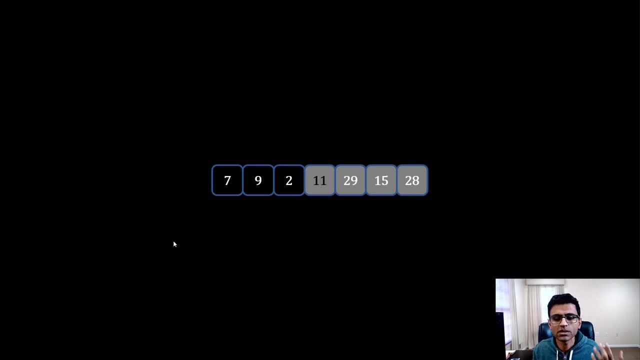 side, we repeat the same process. Imagine you have a left partition and you have a right partition. You have an array of 7,, 9,, 2, and first element, you will consider it as pivot, and then you try to put pivot in its right position. Now we are going to look at how to do that exactly, But for now 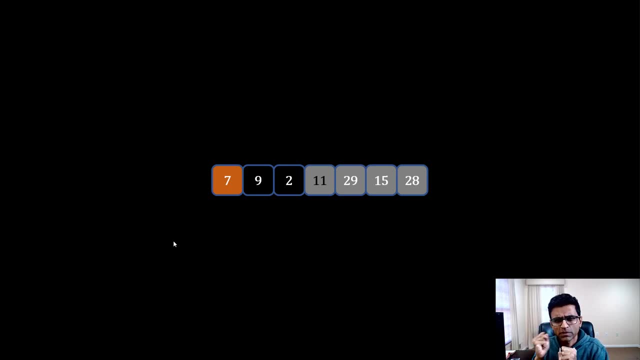 assume we have some way of putting this pivot guy or girl into its right position. So now we put this into right. position which is in the middle and left hand side is elements are less than 7 and right hand side elements which are less greater than 7.. Now we have two. 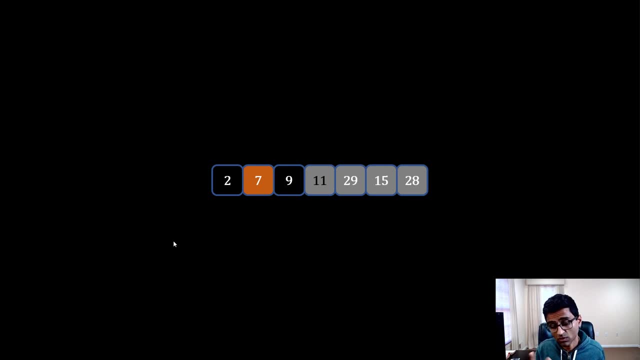 arrays: Left array is 2, right array is only single element, 9.. And when you have single elements they are kind of sorted. So now we can say that 2,, 7,, 9,, 11 are sorted already. So whenever you see gray, 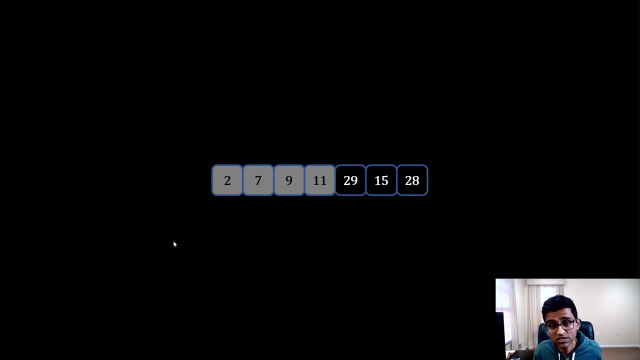 background with black foreground, which means we are done with those elements. We're not touching them. They are sorted. Now let's look at right hand side, which is 29,, 15,, 16,, 17,, 18,, 19,, 20,, 21,. 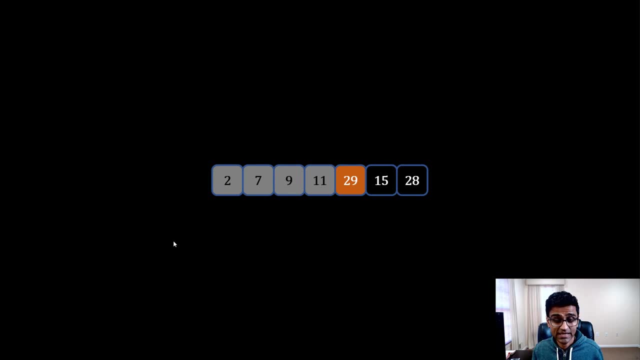 15 and 28.. Again, we will say: 29 is pivot and then we'll try to put pivot in its right position, which is here Now. this created a left and right partition, but right partition has nothing. So there is only one partition, which is left hand side, which is 28 and 15.. Again, we repeat the 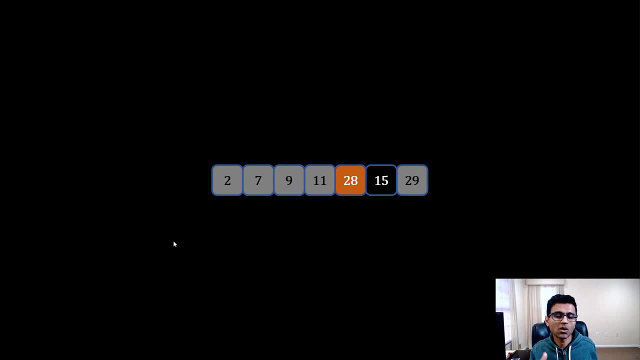 same process recursively. You can see that this is a divide and conquer problem. We solve, we sort one element which is pivot, We create left and right hand side of partitions, two partitions basically, And we recursively repeat the same process on these partitions. So that's the reason. 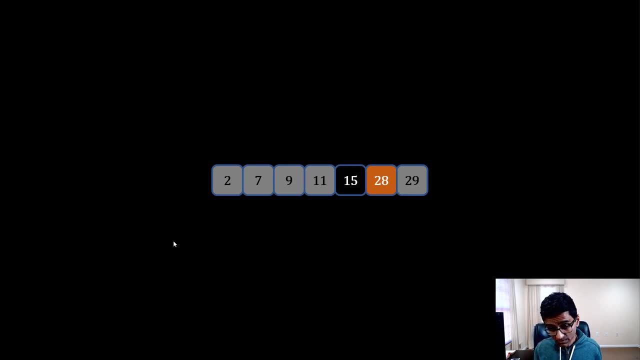 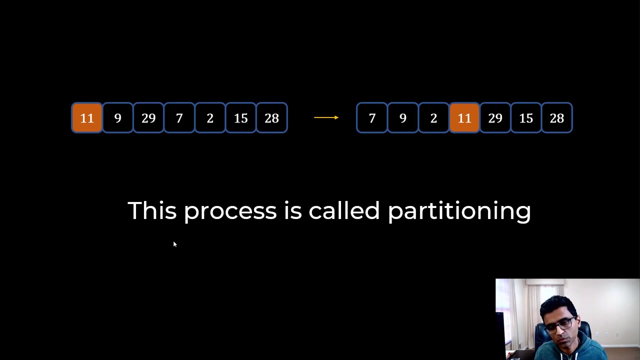 it's called divide and conquer. problem 28 is now in the right position. You are left with only one array, which is single element 15, and that is also sorted. So this way, all array can be sorted. Now, going back to how we can put a pivot in its right position, This: 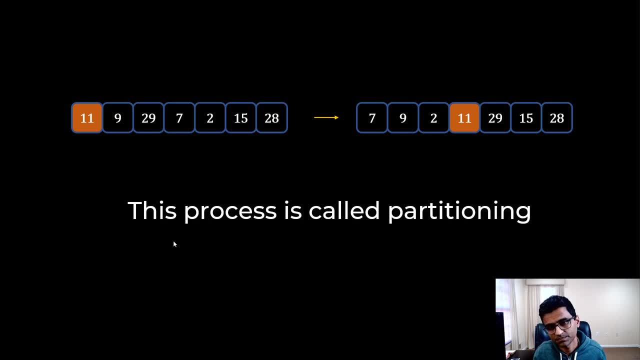 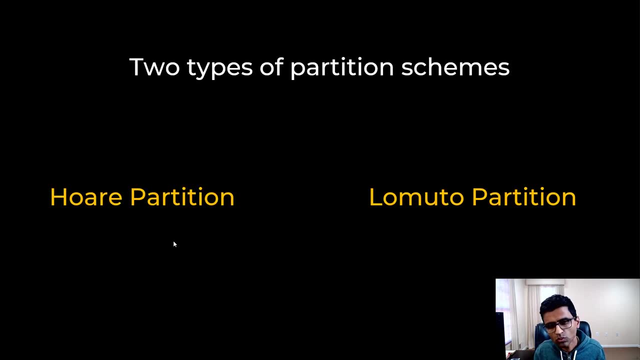 process of putting a pivot in a right position is called partitioning. When you put an element in its right position, you are creating essentially two partitions left and right. And there are two famous partitioning schemes: ORA partition and Lomuto partition. ORA is a British scientist. 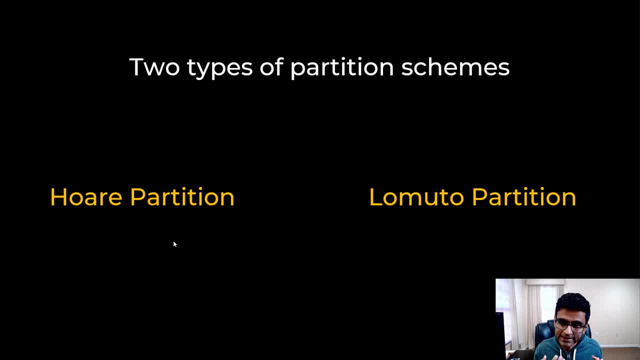 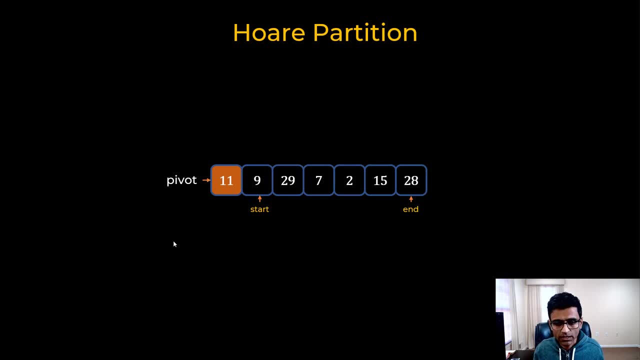 invented quick sort and his original partitioning scheme is more popular. so let's look at that. in here we come up with two pointers, start and end. so pivot is my leftmost element. sometimes people use different positions as a pivot. even in Lomuto partition you will see our people use either leftmost element. 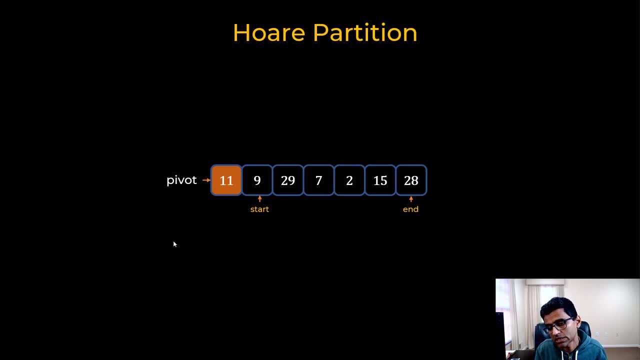 rightmost element or even a median element, medium, medium element as a pivot. but here we are using the leftmost as a pivot and now we have start and end pointer, so we'll first focus on start pointer. that's the reason. my end pointer, you see, it's a gray now, so let's focus on start pointer. so I will keep on. 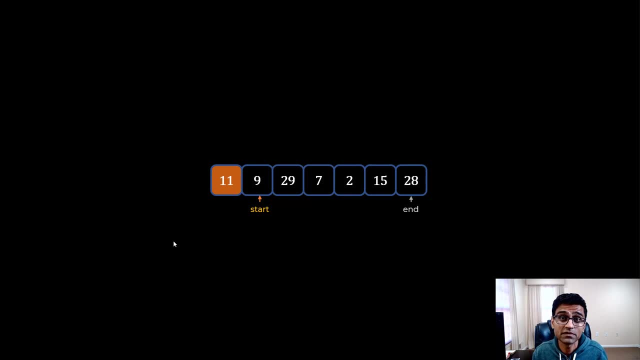 moving start pointer until I find the start pointer, and then I will keep on moving until I find an element which is greater than 11. so we are going through this elements one by one, comparing them with pivot. remember that's important. you are comparing the elements with nothing else. 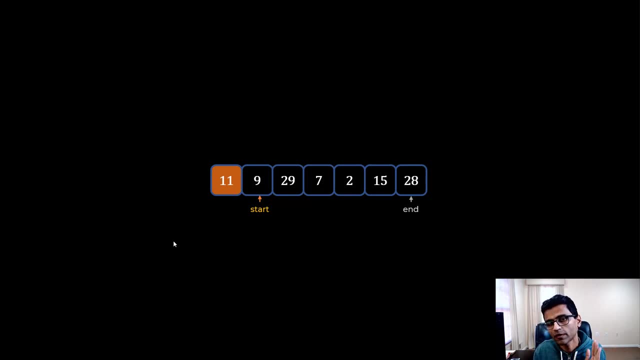 then pivot and you keep on going till you find an element which is greater than 11. so 9 is greater than 11, no, so then you move on. 29 is greater than 11, yes, so then you stop now. now let's focus on end pointer. so my start is gray, my end is amber. I will 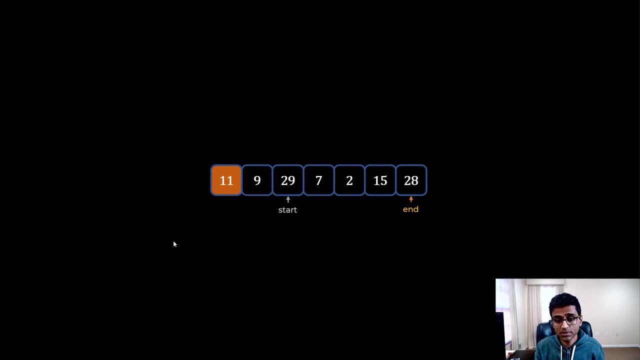 keep on reducing, end till I find an element which is less than 11. so 28 is less than 11. no, so let's move. 15 is less than 11. no, let's move 2. 2 is less than 11, yes, okay. so now my start and end pointers are stopped. all right now. 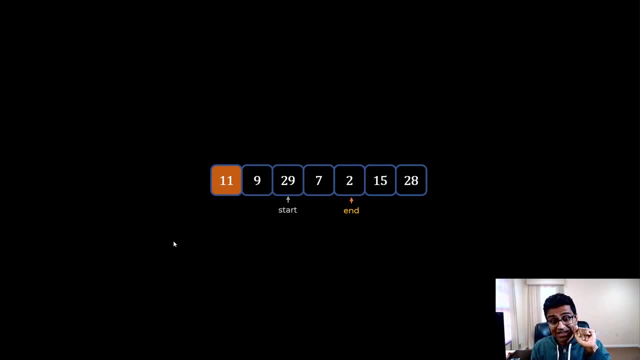 something interest is interesting is going to happen now. we found on the left-hand side element which is greater than 11, a right-hand side it is less than 11, so we can literally swap them, because the entire purpose of quick short is you want to put pivot, which is 11, in a in a place where left-hand side. 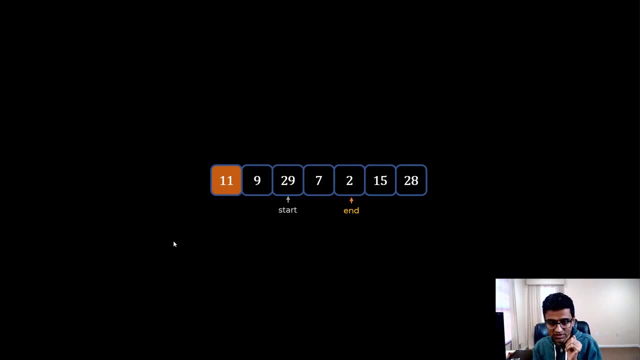 is all less elements. right-hand side is all greater elements. so swap it. when you swap it, you get this. now again, you repeat the process. after you are swapping. done with swapping, start the same process again. so we start with start pointer now and start pointer we move from 2 to 7. because 7 is still less. I still want to move it one more so. 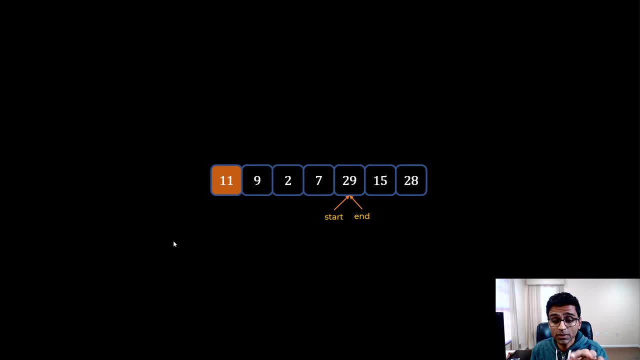 remember the start pointer will keep on moving until you find an element which is greater than 11. so 29 is greater than 11, so now I will stop my start. so now I will stop my start. so 29 is greater than 11, so now I will stop my start. 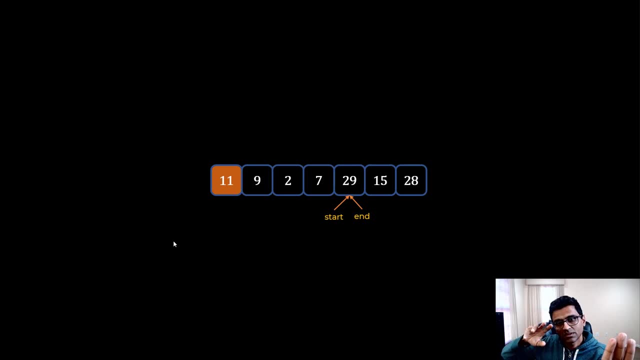 now let's start with now. let's do the iteration for end pointer for end pointer. what is the rule? the element 29 is greater than 11, so then move. so now I moved and I came here. now. we stop this process whenever and will cross the start. 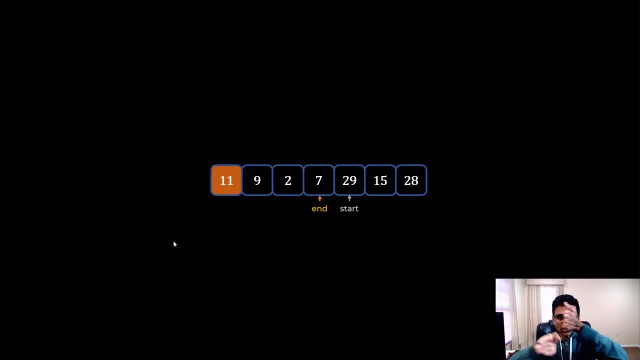 you know, there is a start, there is an, and when n crosses start, here you stop. when you stop, at that time swap your end and your pivot. something magical happened now. well, 11 is in its right place. see, this process is? it sounds complicated, but it's. 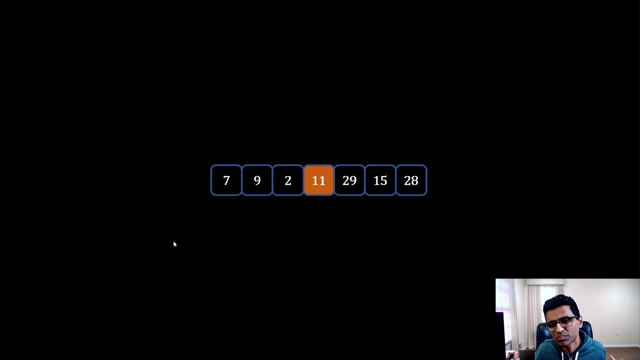 not. actually, all you're trying to do is put this 11 element in its right position and then you do the same process for left partition, right partition, and if you keep on doing that, the whole array will be sorted, as we saw in the earlier presentation. so this was. 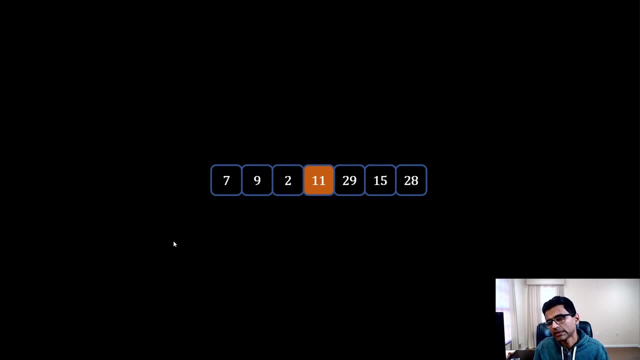 Hoare's partition. this is very popular. there is Lumoto Lumoto partition- I don't know how to pronounce it, sorry, Lumoto partition. the way this works is you decide your end element as your pivot. you can decide your left element or middle element as well, but here the end element. 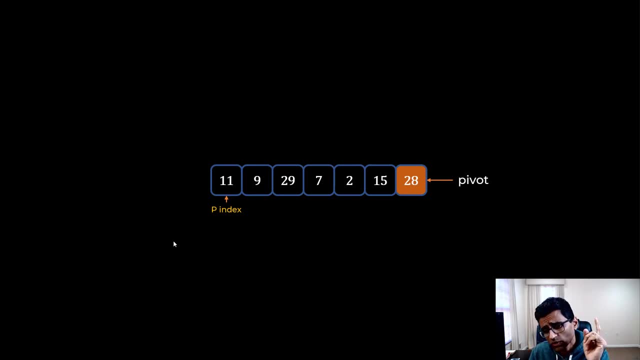 being pivot is very popular, and then you start element which is 11, you call it p index, which is partition index, and you keep on moving partition index till you find the element which is greater than pivot. see now I found 29. see, I was 11. 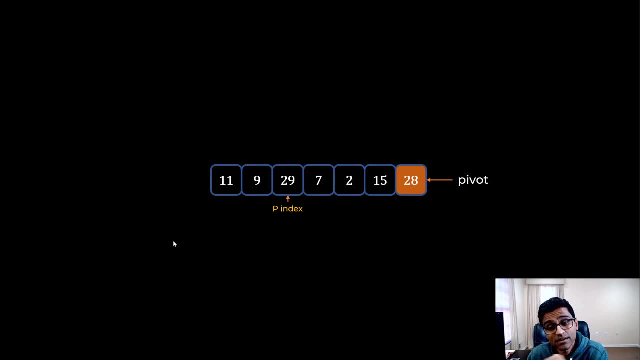 then I move to 9 and then 29. see, now I found 29. I was 11, then moving to 9 and then 29. now 29 is greater than 28. okay, so again just to remind you, in this whole partition process we compare every element with pivot. we don't compare it with anything else, with pure. so 29: 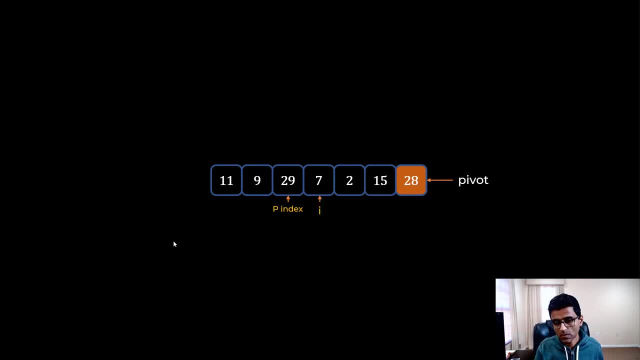 is greater than 28. that's why we stopped. now we start another counter called i and that i starts with p index. so i initially is same as p index. it will keep on moving until it finds the element which is less than 11. so 29 is not less than 11, so it will move and it will come. 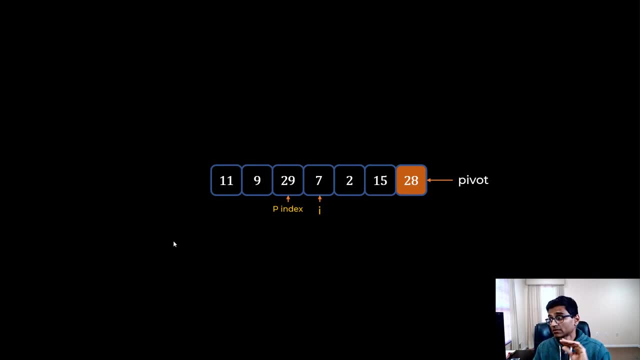 here and now, 7 is less than 11. all right, now something interesting is going to happen. let's stop here, let's do something interesting. what is that? so now, at this position, you swap 29 and 7. so when you do that, you're creating a left hand side which is less than 28. 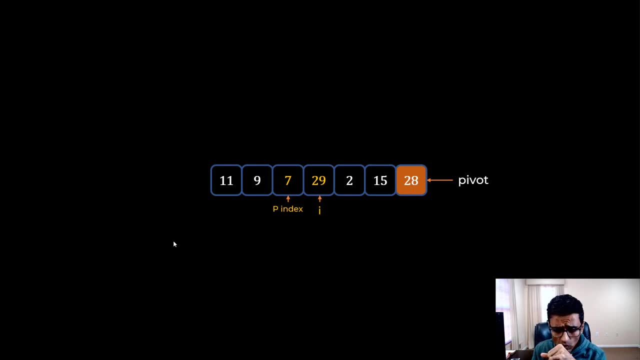 right hand side, which is greater than 28. okay, now let's move on. so now p index. i will move. so the rule for p index, friends, rule for p index is this: you keep on moving till you find element which is greater than pivot. so p index is 7 right now. it is not greater than pivot, which is 28. 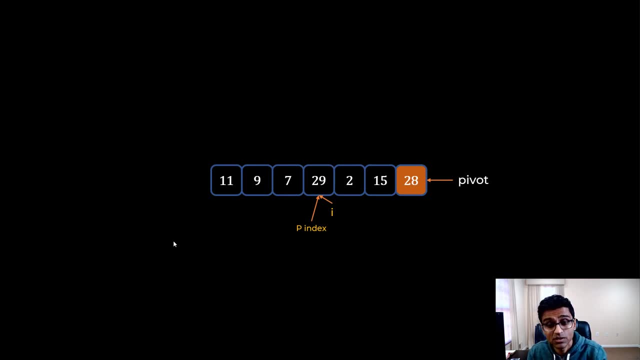 so you move. now you came to 29. 29 is less than 28, so stop, so 29. stop so once you stop p index, then you worry about your i. so i is a counter and the rule for i is reverse: you move i till you find the. 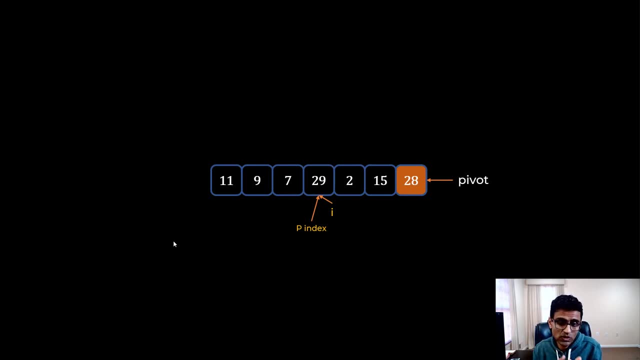 element which is less than pivot. 29 is greater than pivot which is 28, so i will move it. so find 2 which is less than pivot. now, stop. whenever we stop, what do we do? yes, we swap. so now we swapped it. perfect, again repeated. oh my god, this repetitive process is boring, but 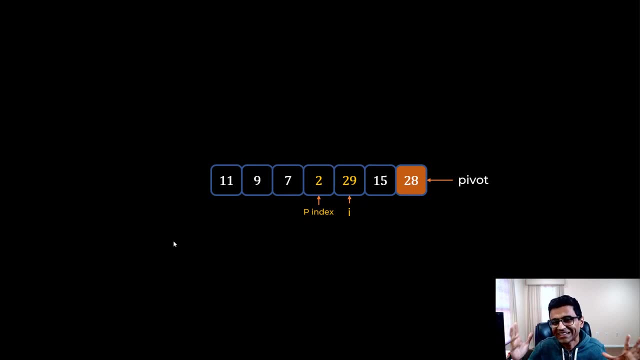 this is the art of computer algorithms. it makes things efficient. so p index- again. i move till. i find an element greater than 28, which is 29. so again, p index will be stopped here. i i will move till. i find the element which is less than pivot, which is 15.. 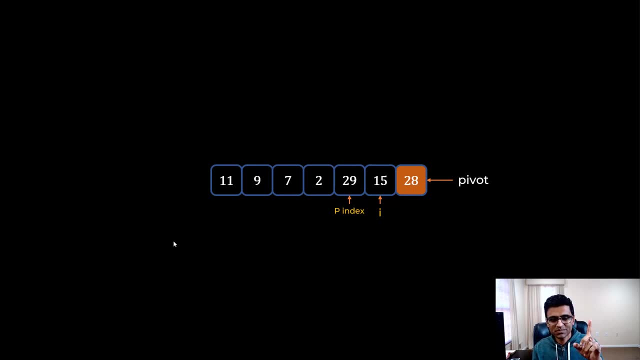 and whenever we stop, what do we do? we swap: see 15, 29, i swap, they change the position again, repeat. so p index 15, you go to 29, again you stop, i, you go to 28. so that is less, all right, man, i'm tired, all right. and whenever it is less, what do you do? you switch p index and i. 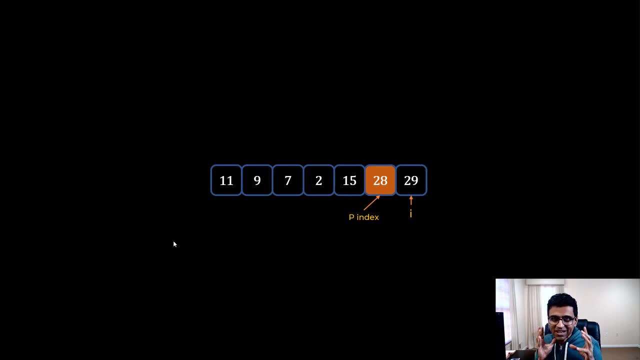 now you switch at this position, you realize your 28 is in a right position. 28 was our pivot. now 28 is sorted. it is in right position, which means all the elements on the left hand side are less than 28, all the elements on the right hand side are greater than 20.. 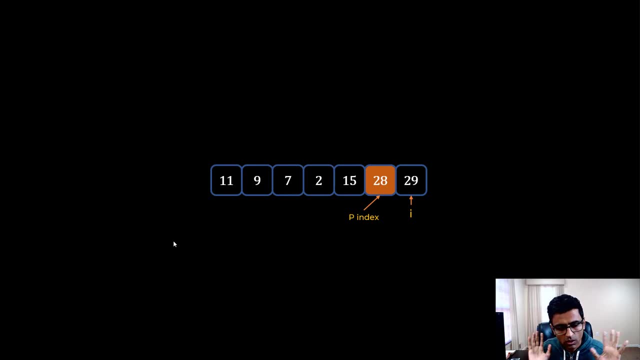 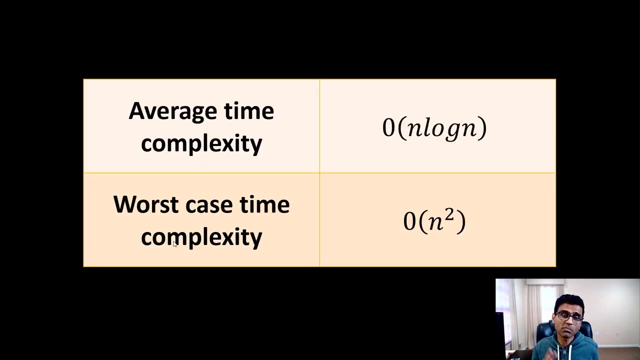 this was lumoto, lumoto, lumoto partitioning scheme, i don't know how to pronounce it. how about the bigger complexity? the average complexity of this algorithm is n log n, because, if you think about it, if you are partitioning in less equal portions every time, the source space for left hand side, right hand side, is reduced by two. that's why 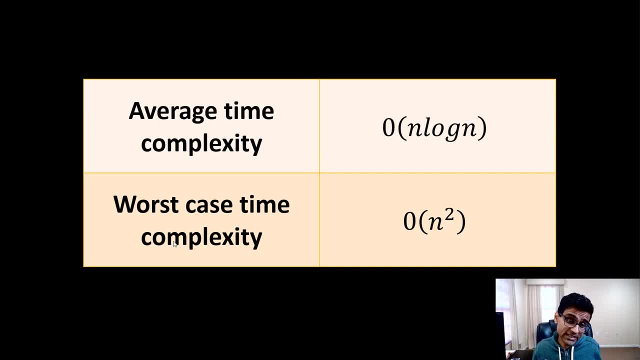 it's order of log n. worst case time complexity is order of n square when your list is already sorted. if the list is already sorted, uh, you will create very imbalanced partition, which is you will have either left-hand partition or right-hand partition and you're not really effectively reducing the search space. so for 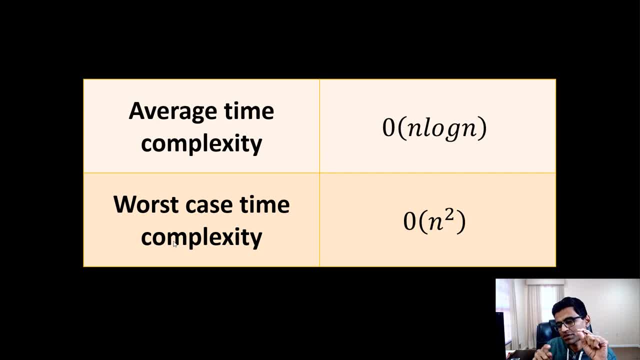 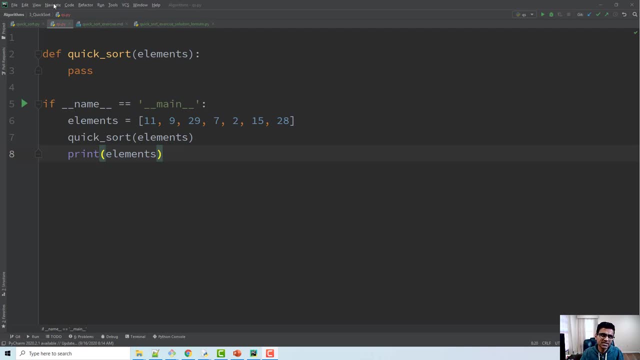 each element. you are performing an, an iteration, and you have n elements in total. that's why it's a order of n square. let's write python code. now we are going to implement quicksort using hoare partitioning scheme. in pycharm, i recently discovered this awesome mode called zen mode. 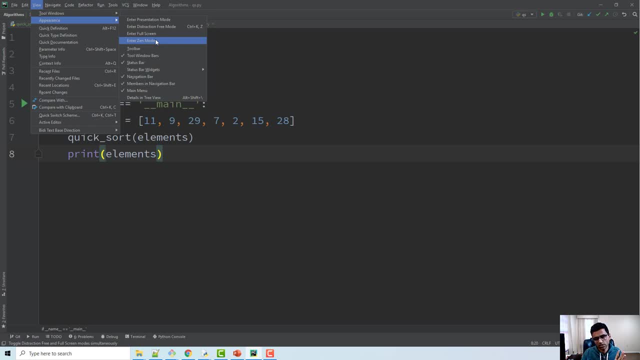 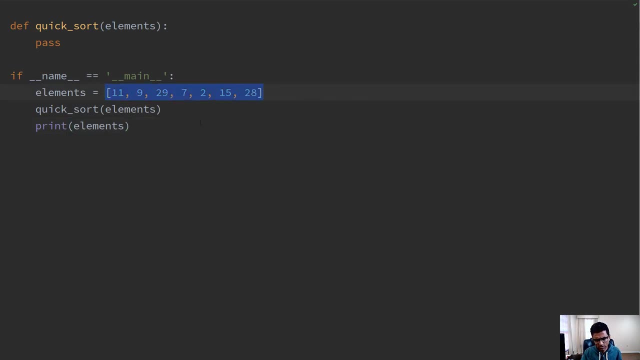 where you literally enter- kind of like a distraction- free full screen mode, so i'm going to use it here. i have this list of numbers which we saw in the presentation and i'm trying to sort them. so the first thing we saw was the 11 was a pivot, and let's try to put 11 in its correct position. 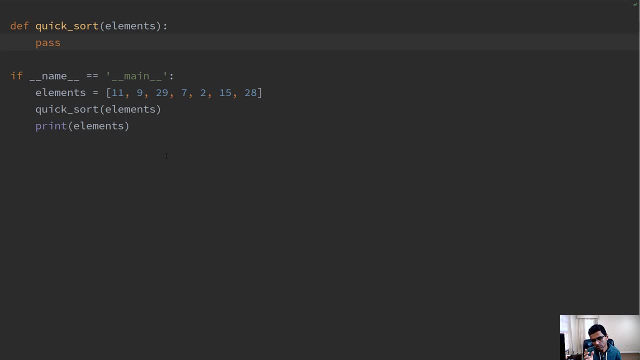 okay, so that is the first thing we are going to do, and that is called partition, actually. so when you do partition, let's do this partition. so i'm writing a partition function, partition, and once this function is done, i should have 11 in its correct position, which is almost in the 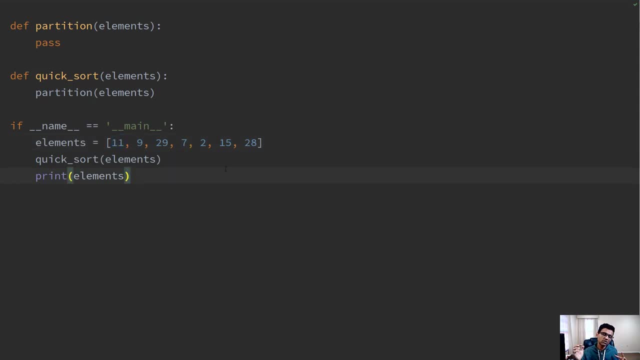 middle of the list. this is the common approach of programming, which is you try to small, solve smaller problem first, and then you evolve and you build your logic on top of it. so for now, in my brain, all i'm thinking is i want to put 11 in its right position using the partitioning scheme, and i'm 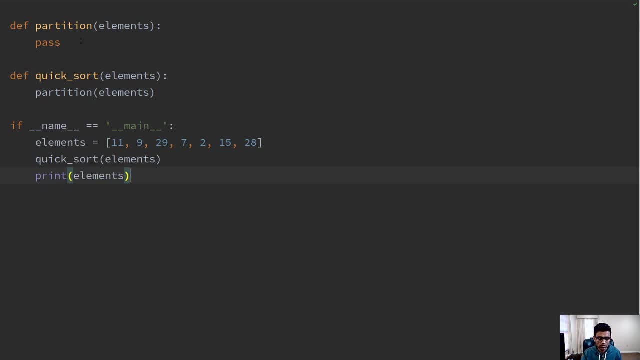 using this system, which is called systemData, to do that. so i'm just going to show you how to do it. so let's go back over to the windows, and this is one example of the systemdata. so i'm going to show you how to do this systemdata, and in this systemdata we are going to create a statement. 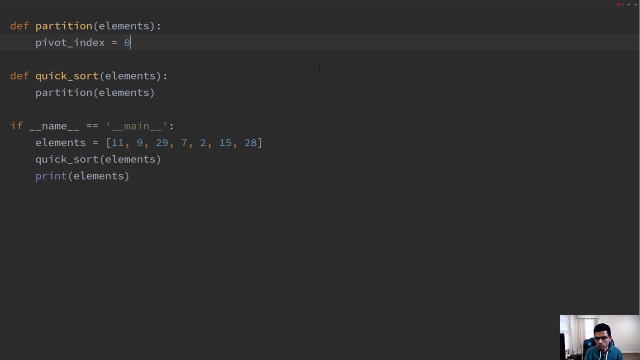 function which is known as the pivot index, and what is pivot? that means pivot is a constant index, and that is why the symbol pivot is second and the winning plus is the pivot index. so if you create a pivot index in a set of these two items, you're going to get a pivot index that is 0- uh, i'm going to put that into this゠. and then the pivot index is basically this. so first i will say pivot index. so right now, the pivot index is zero, okay, and pivot is basically this. 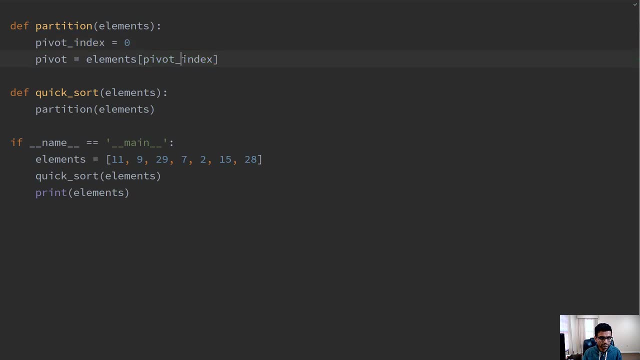 is basically this, or let me just do this, yeah, or this, whatever, all right, so I'm just using variable, doesn't matter. and here we saw that we want to start with this pointer called start. so start pointer is nothing, but what is it actually? so start is pivot index, pivot index plus 1 right and end is basically you. 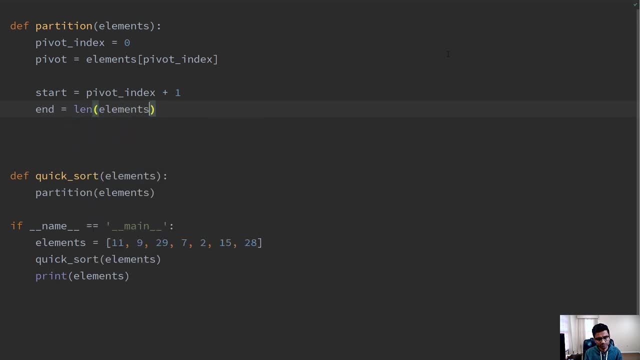 know your last elements and then, first you want to start with start element and you want to move till you find a place where the element is greater than 11, so I can run, maybe while loop. okay, so while element of start is less than equal to pivot. 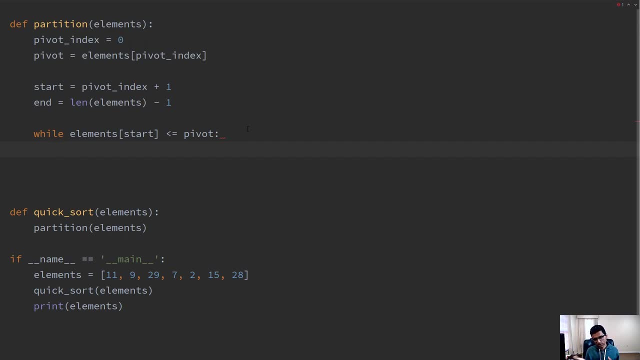 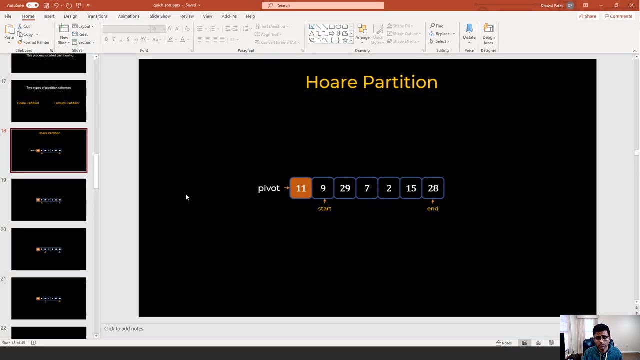 sometimes you might have duplicate elements, so I will just say equal to as well, and you just, you know, keep on incrementing it. if you remember our presentation, friends, uh, where is our presentation? yeah, here see, what we did is. we were here and we kept on going until we found 29, which was greater than 11, and then we stopped. 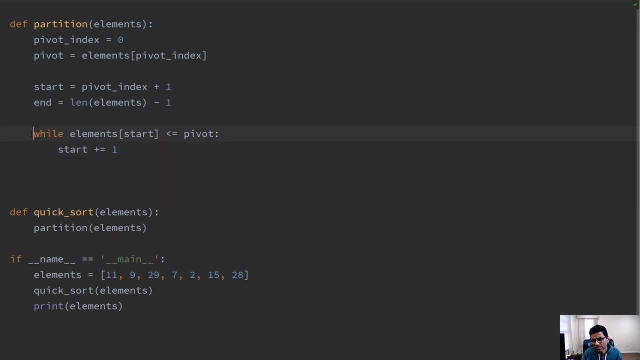 so that's exactly what we did here. you know, we went through all the elements till we find something which is greater than until, if it is less than equal, to keep on going, but then you stop. also, what we do is now same thing for n right. so while element n, if the end is greater than pivot, 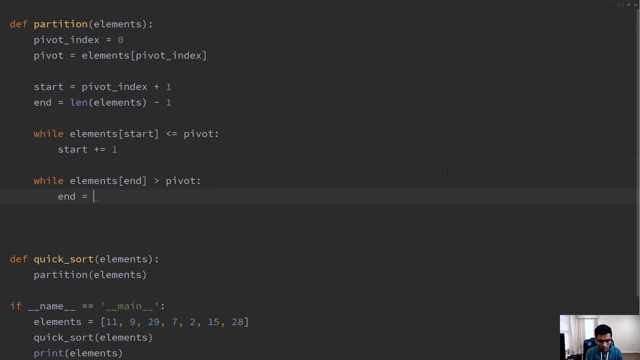 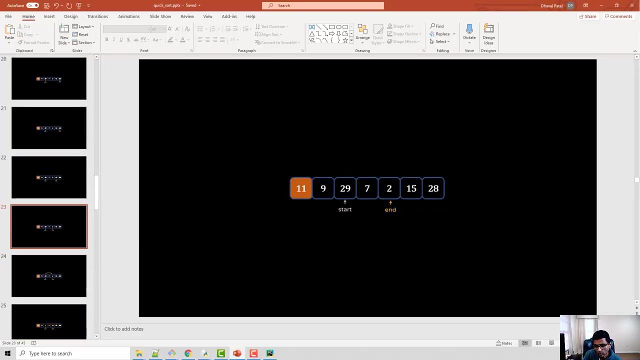 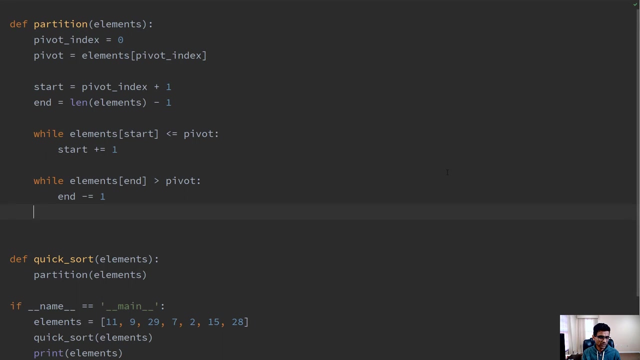 you keep on going. which is n is equal to n minus 1.. this is a short way of writing it, okay, so we will now stop here. so we'll start with n and we'll stop here. so when we stop now, we want to swap those two, start and end. so here, at this point, you just swap start and end. how do you? 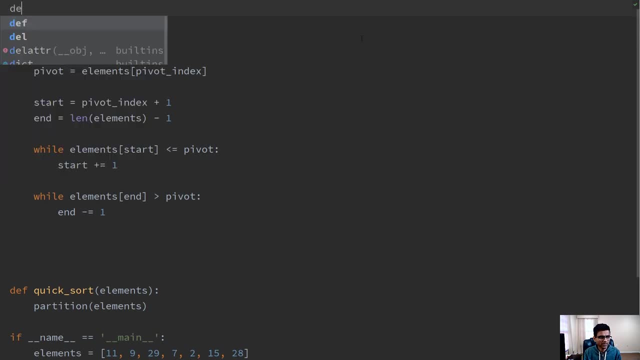 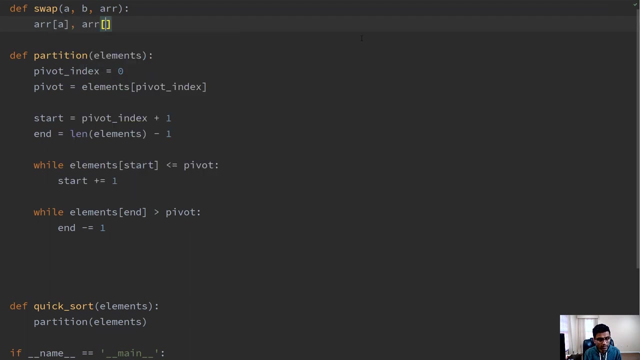 swap them. well, we can write a simple swap function for that. so Python allows you to do swapping in an easier way. you can just say: a of B, elements of i, comma, elements of J. okay, let me write it so you can actually do this. you can do this, uh, it will work, but just to make things more primitive, you know, I will just say: 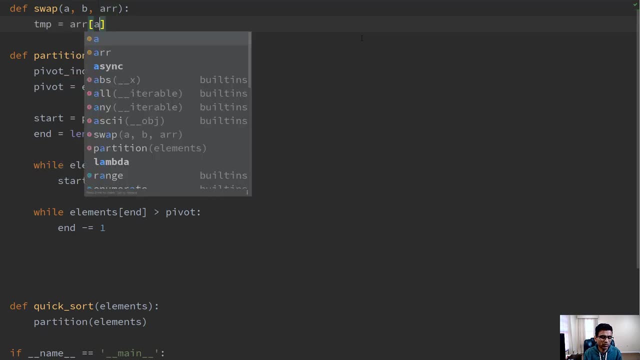 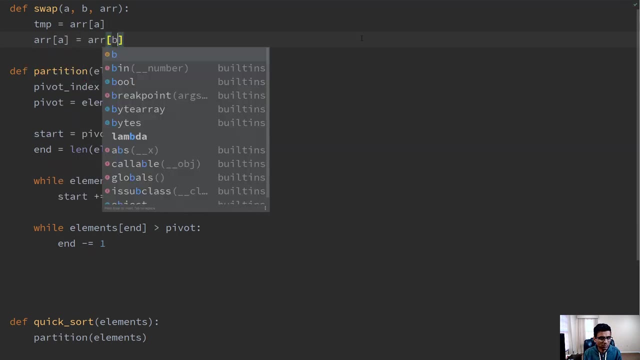 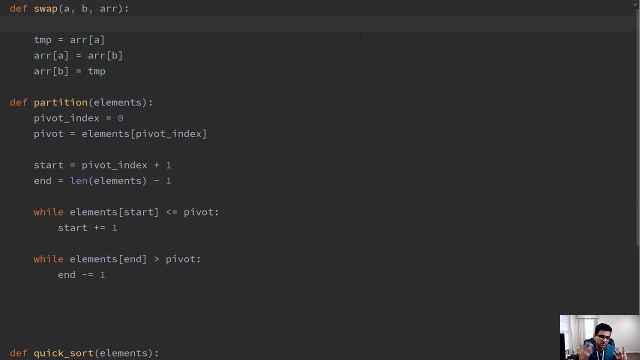 okay, I will use the old school temp variable method. you store first the first element into temp, then you say this B, and then B is equal to temp. this is a standard way of swapping elements in any programming language. and just to be in on a store side, if a not equal to B, then only do it because I don't want to. you know, if they are both. 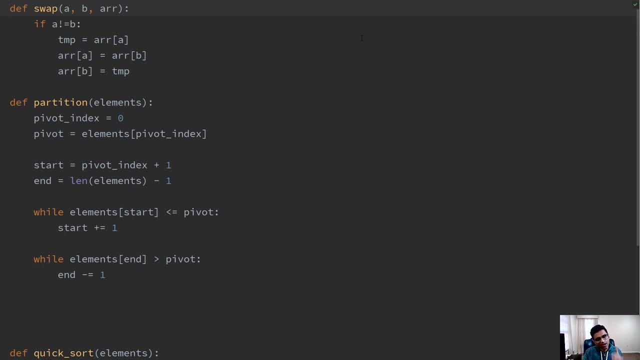 same index. I don't want to swap it. okay, now we are swapping what? okay, we are swapping. start and end, simple. there is no rocket science here. guys, guys and gals, there is no rocket science. and just to be on a safe side, I want to make sure, if 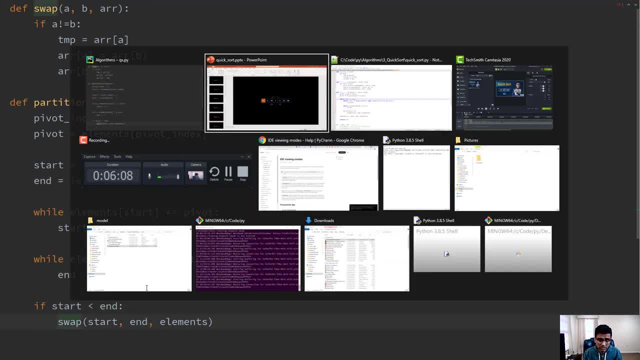 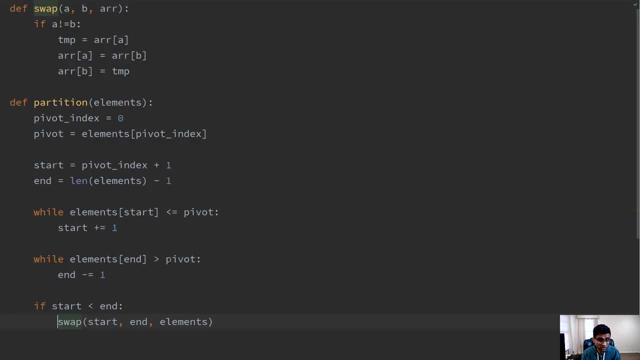 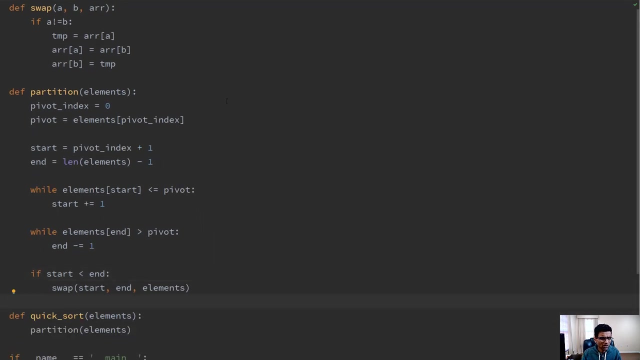 start is less than n because, see, you will stop this when n becomes less than start. you don't want to perform any exchange between start and end when n is less than start, or you know, so you swap it if start is less than n. so far, I hope it makes sense to you all. this is the code, and when I run. 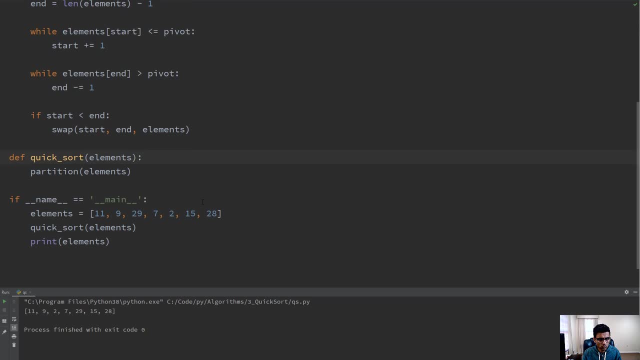 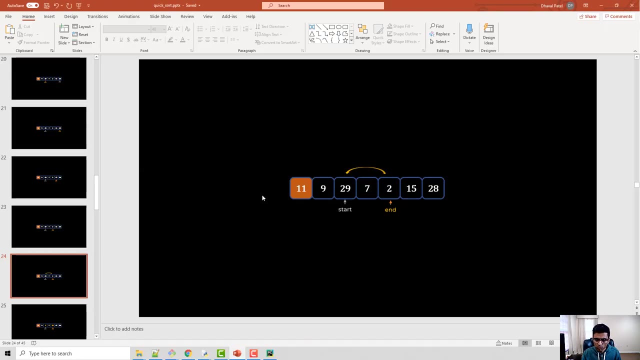 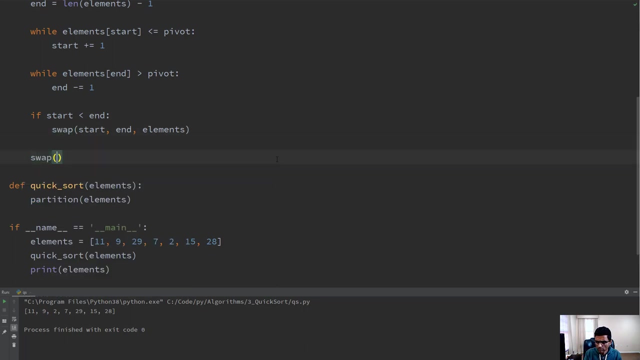 it right click run. oh, we forgot to do one thing actually. uh, remember, once we come to this position, we want to swap. end with pivot, so let's do swap. what do we want to swap? and with pivot? okay, so swap pivot index with an in elements array. and when you run it, you find that 11 is- oh no, 11 is not in a correct position. something is. 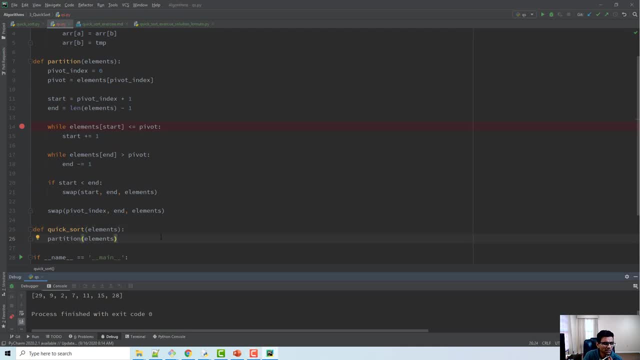 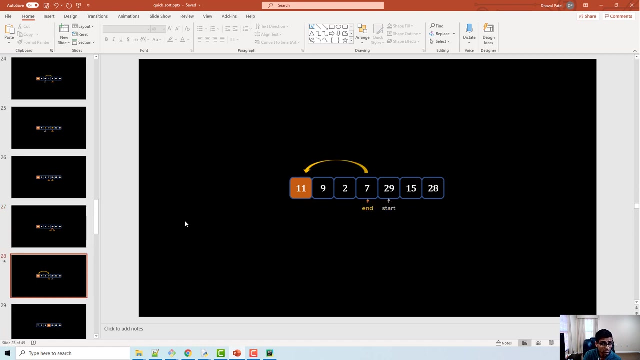 going on. okay, after code examination, I'm finding it that we are running two while loops. okay, which is start and end, but remember we need to run an outer loop as well. so when you swap between 229, we have to keep on going till and crosses the start. you know start and end, then if and crosses 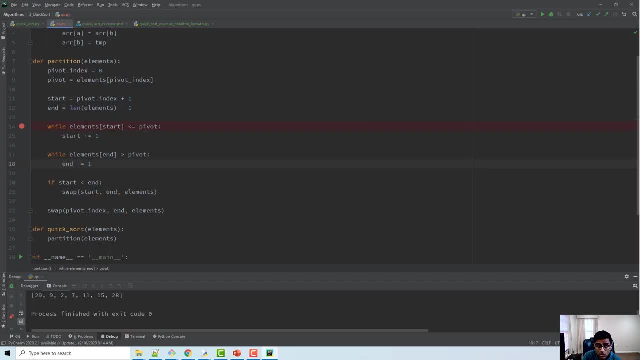 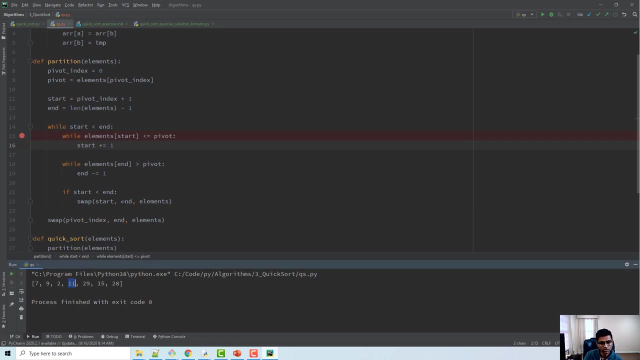 the start, you have to stop it, so there has to be a outer while loop as well. so while start is less than- and this has to be there, okay, and when you right click run 11 is in its correct position. let me enter my Zen mode. enter Zen mode. 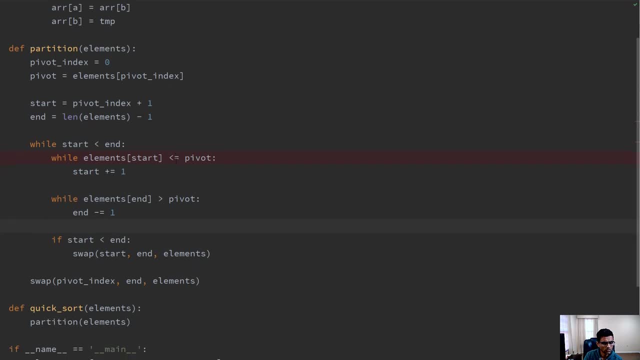 enter my Zen mode. okay, I'm meditating now. so my partition function looks good. I need to now make it generic. I did, uh, pivot handling for the first element. I need to now do it recursively. so how do I do this recursively? well, hmm, let's see, there is something in partition element, so I need to first here, pass, start and 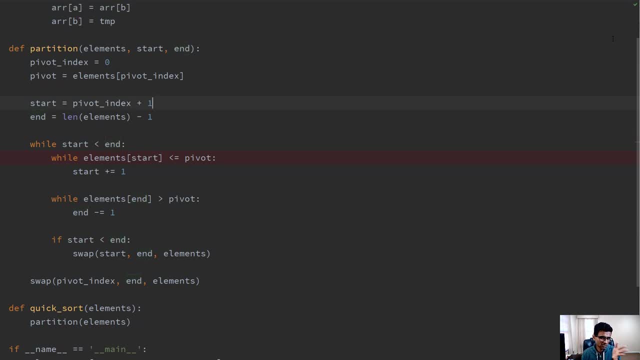 end element. you know I was taking this as a hard-coded values, but this has to be made an argument and this will be start correct. so now partition should be start and end. start and end. quick shot should also have start and end because it's going to be called recursively and start and end will be when you call it for. 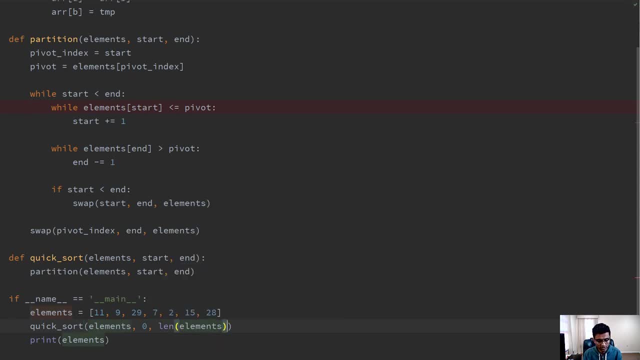 the first time, it will be length of elements minus one, because list starts with zero index. that's why we do minus one. and, hmm, now we do this, which will work, but in the end, uh see, when I put 11, it's in its right position like this: 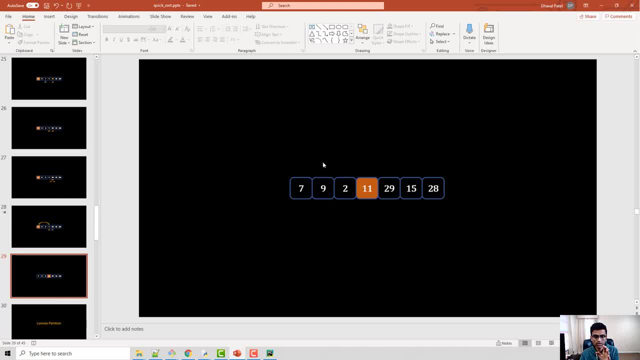 I need to now recursively call quick short on left partition and right partition. so, whatever position I put this in, I need to return that index. let's say this is a partition index, so that index, by the way, will be what see index will be end. so end pointer is pointing to that right position, so that is the position. 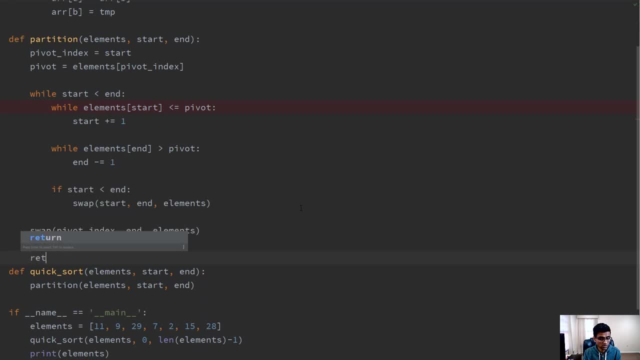 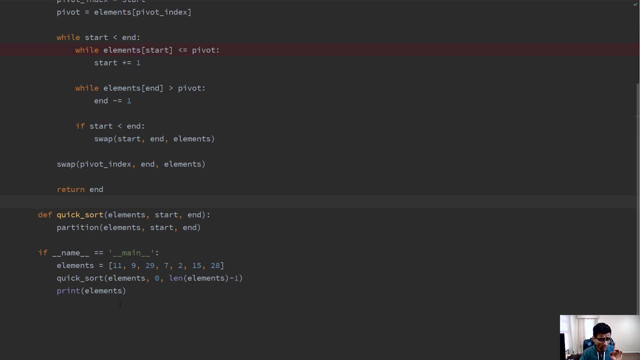 this is end, so I need to return and here, so I am returning n. okay, and that I will call it a partition index, and once I have a partition index I have two partition. so this is the API partition index. I need to Now Recruit version and now we have the data of the project that I need to really copy and paste that in, and after that I need to. So just keep having IO and 유 and we also need the data of all these applications murdered. so we're going to safely copy and paste it and just egg it on to the external vendors. it's now up to the Element can replace it and we're going to be time and production. now I need to review order, so I need to props the virtual'm getting started, so open tm file. now I need a machine change or you have. 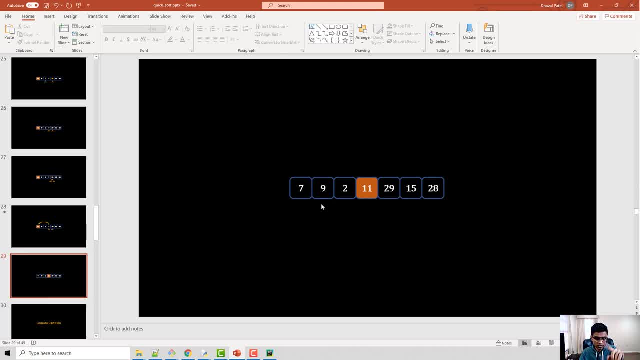 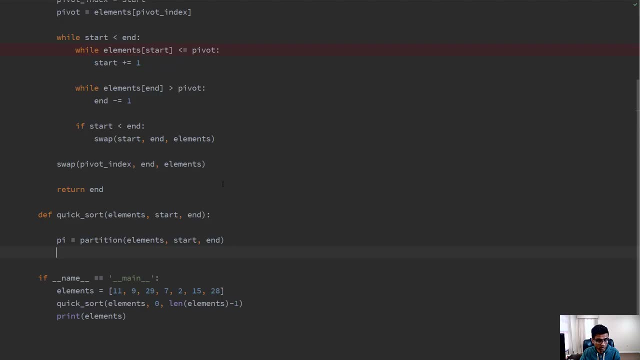 call quick short on left partition which is starting from 0 or start position, to this partition: index minus 1. okay, so I will be doing something like this and I need to call it on P I index plus 1 and end as well. I hope this makes sense. this is a left. 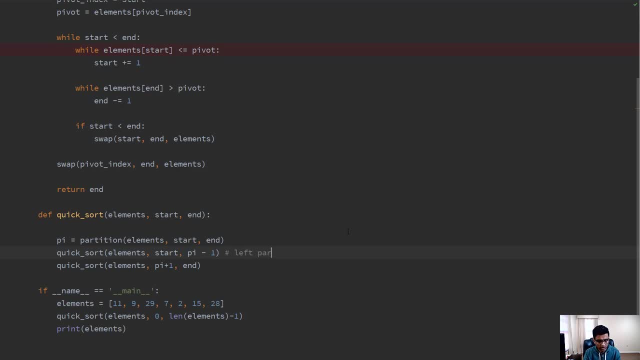 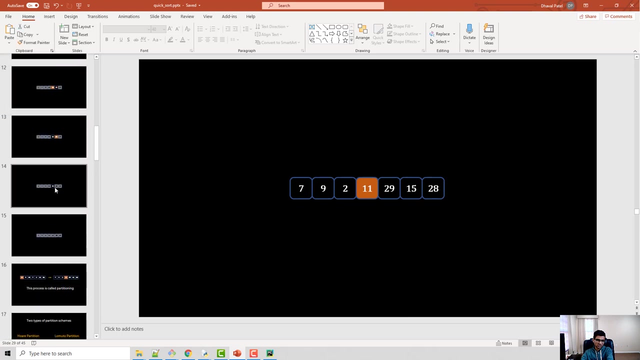 partition: okay, left partition: this is a right partition. and how long should I do this process? well, if start is this, then end, because eventually, like if you look at the initial presentation here, you will get elements which will be like start and end will, let's say, if you have one element, the start and end points to same. 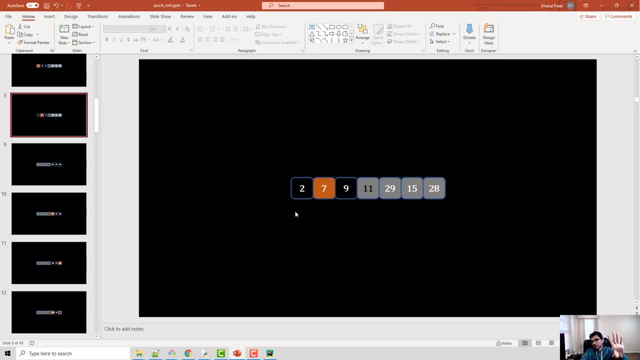 position. let's see you're just two in your array, then start and end. if they're equal, you want to stop it because that array is already sorted. there's a little bit of a thing here. but if you are looking at the Marly's, there's a little bit of a thing here. but if you are looking at the, 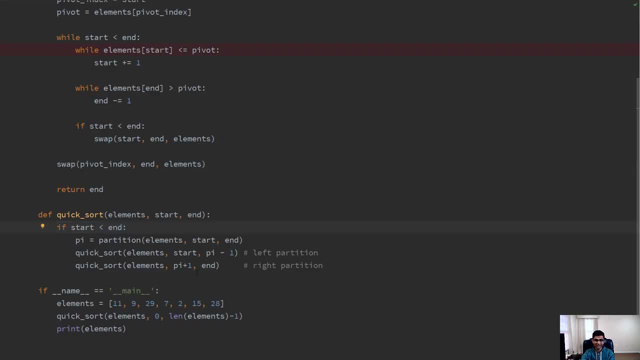 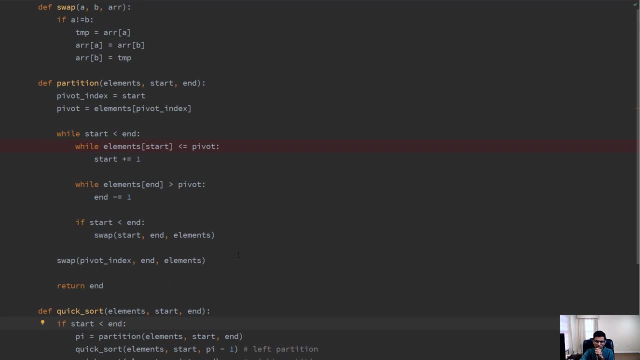 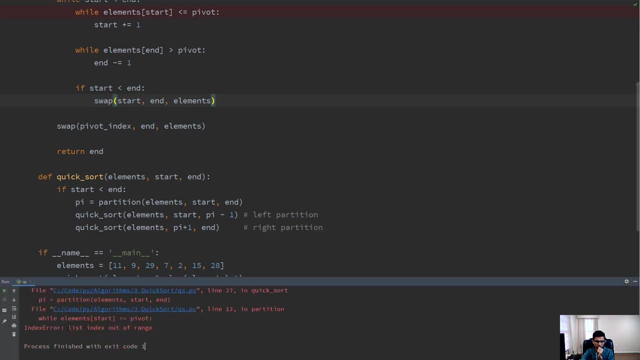 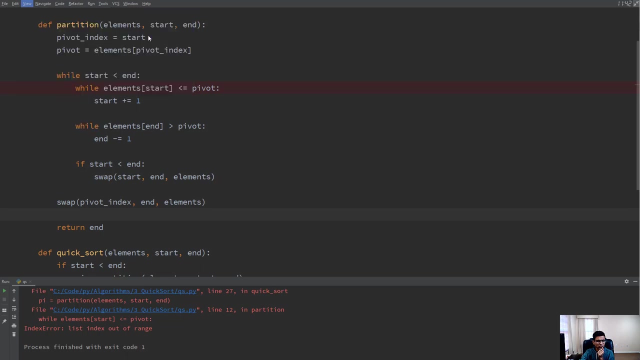 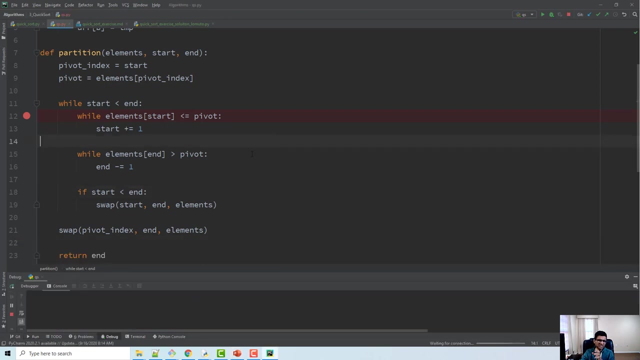 why I have this condition. if start is less than and- okay, all right, let me just quickly verify. everything is okay. all right, looks good. right-click run: okay, list index out of range. that is the error I am getting. okay, let me come out of my meditation. exits and more okay, so right-click debug: see this debugging. 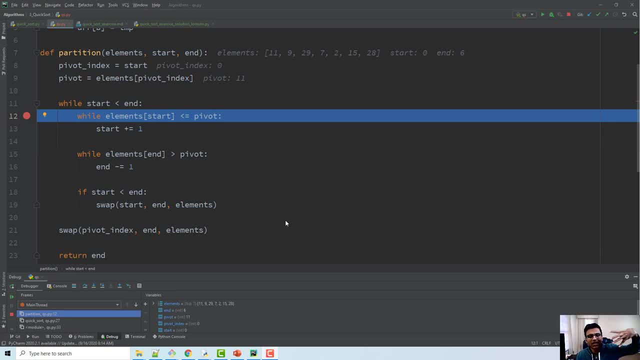 thing is very useful whenever debugging allows you to go deeper into your problems, as if your surgeon is performing a surgery and doing a little investigation. so you want to know why we got that and that error. okay, so when you do this, you will have this variable window where you can see the elements. 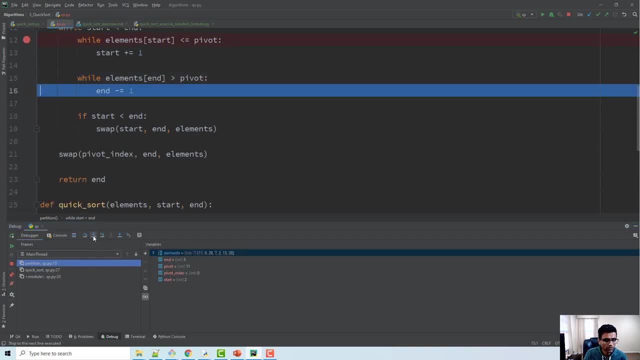 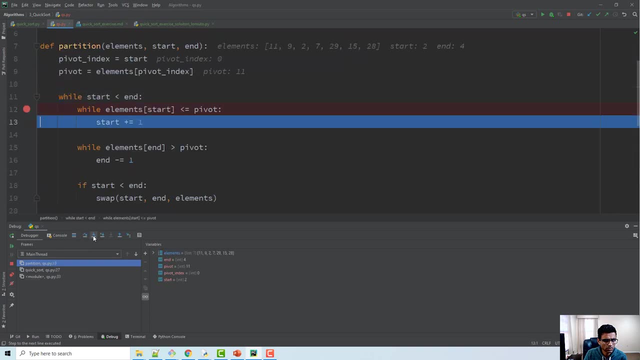 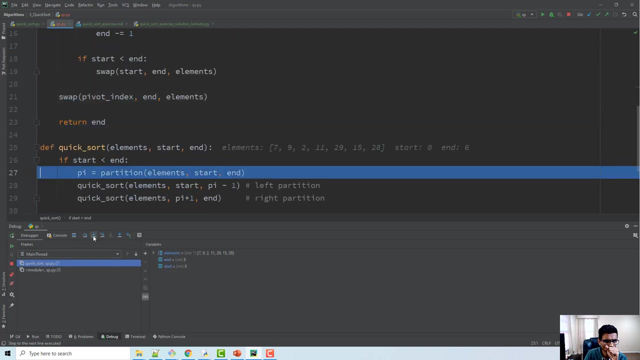 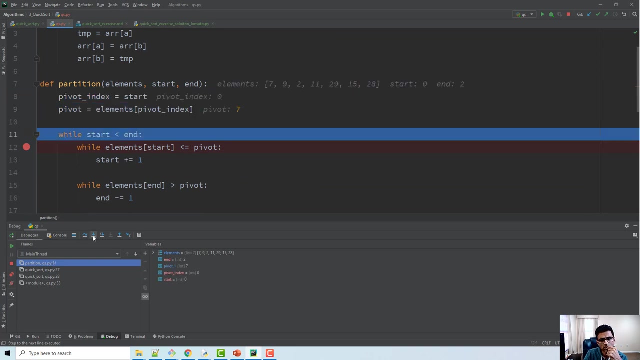 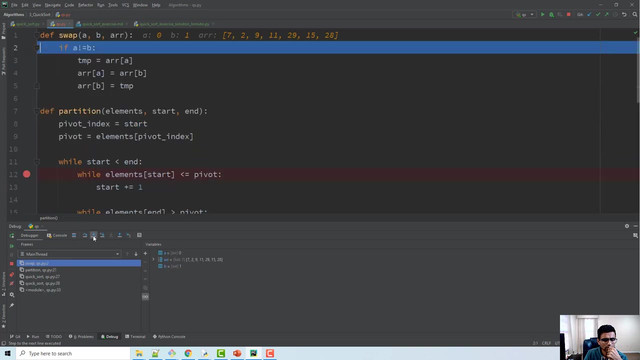 your local variable state and so on. so I will just okay, this one looks good, all right, so let's go ahead and do this. so my start is zero and this is n okay. I keep on going and you have to be patient actually to find out the problem. 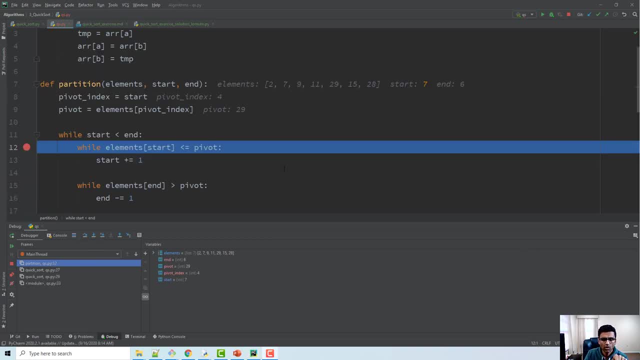 okay, I find the problem- see what's happening here is: the total number of elements is: see one, two, three, four, five, six, seven. so your index could be at most six, and I'll start here. he just keeps on incrementing when we are solving a problem. for this array: 29, 15 and 28, see the element 15 and 28 is less than 29, so 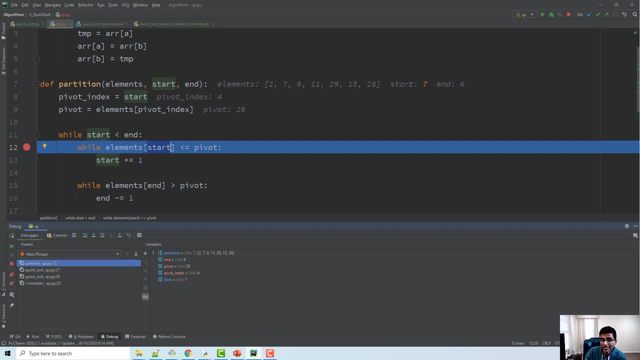 this loops, loop keeps on going and whenever you see element elements in bracket 7, see start value 7 right now is gonna fail because the maximum index that elements can take is 6. so we need to put some type of boundary check here, which is: while start is less than length of elements. 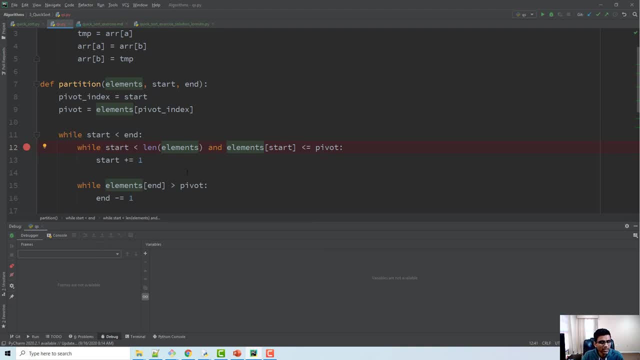 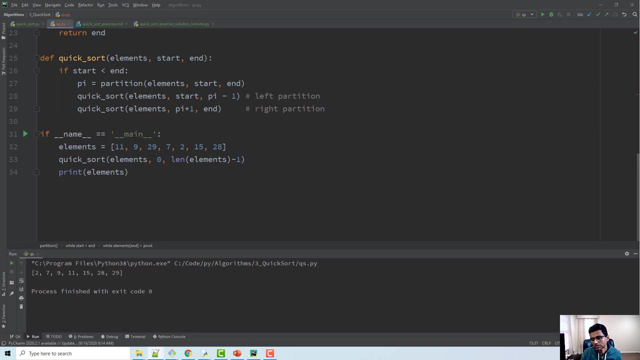 and then we need to get some type of tail Better somewhere. nice, give one type of binaural okay, because this will make sure you don't go out of bounds for your given array- and right click, run. the array is sorted. Beautiful, it is working, friends, it is working. usually when you're writing a 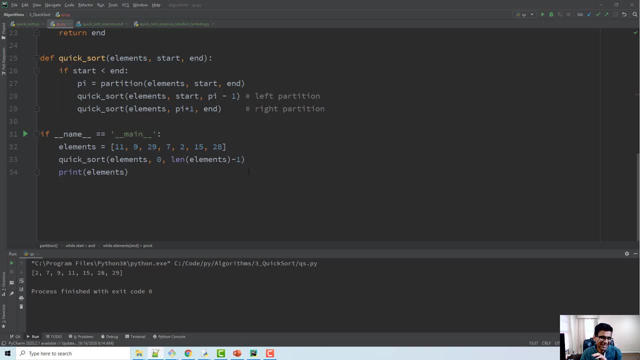 program, you need to write some test cases, and what I mean by that is you need to test for various edge cases. what I mean by that is something like this: let's say, I have all these arrays and you want to sort it, so I have one array which is empty, one which is only. 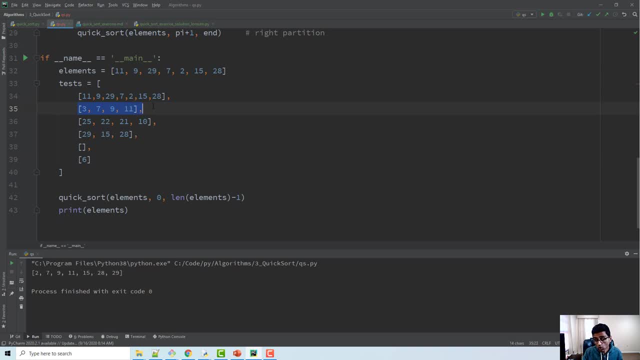 one element. I have an array which is sorted in ascending order. I have an array which is sorting in a descending order. you need to consider all these cases and make sure your program works. so I will run quick short for all these beautiful test cases and make sure it works. and I find that it does work. 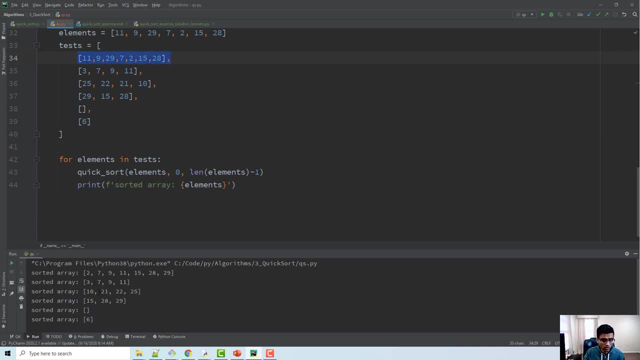 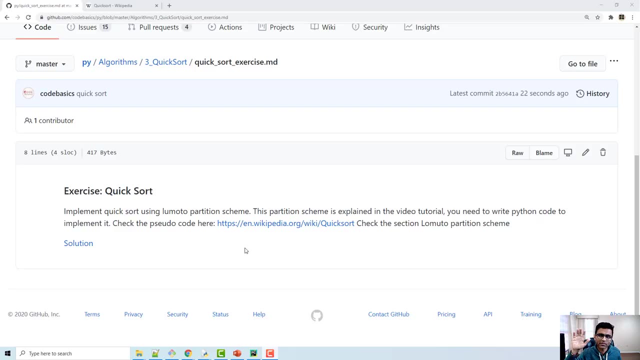 indeed. so you can see that all these arrays, you can just compare. all these arrays are kind of sorted perfectly. all right, our quick sort using who are a partition. you can just compare. all these arrays are kind of sorted perfectly. all right, our quick sort using who are a partition. 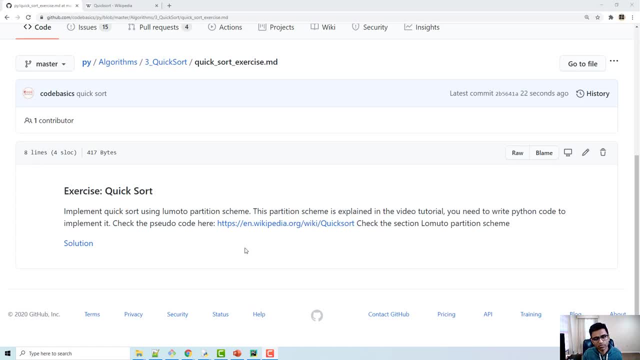 scheme is over. as an exercise, I want you to implement same quick short using Lumoto partitioning scheme. here is the exercise description. you can find the link of this github MD file in the video description below. I also have a link of the Python file which I implemented, basically this particular file, here. I. 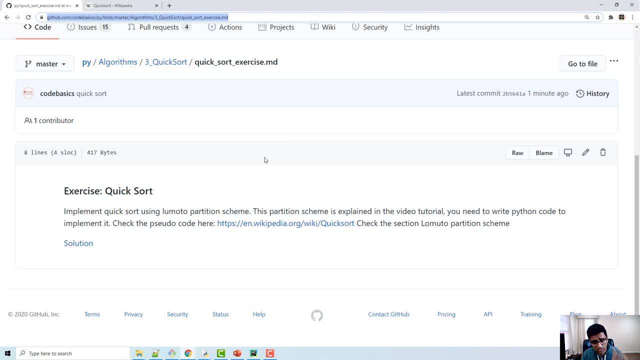 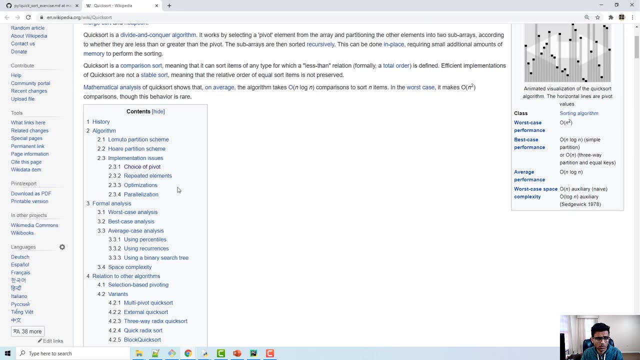 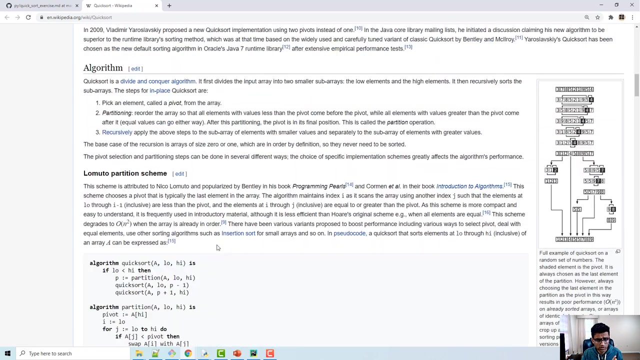 have a link of that in the video description below as well, so check it out in exercise. you can look at this Wikipedia link for quick shot and you can go to the motor partition scheme and study the pseudo code which is mentioned here. so this is a pseudo code and all you have to do is 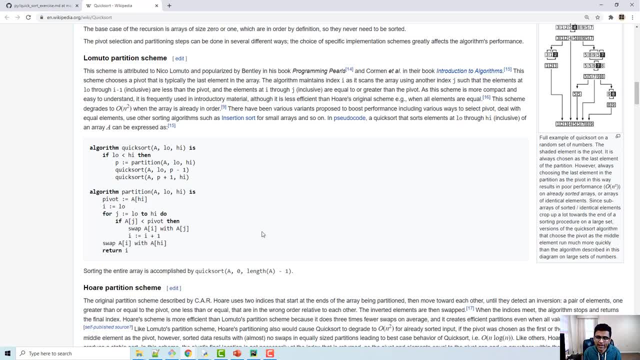 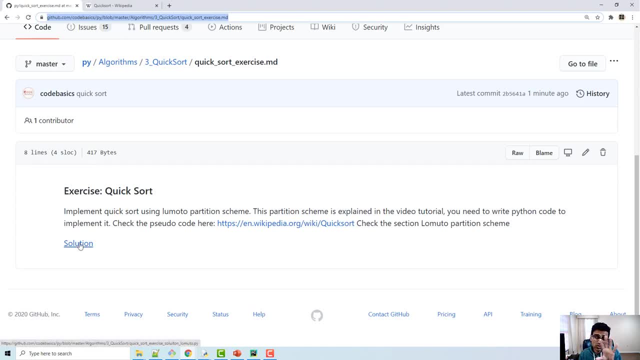 write a Python code for this one. it should be fairly straightforward. I hope you try it on your own before you click on solution link. clicking on solution link directly is going to give you a fever, actually. so be careful, or you need to try on your own. coding is something you have to. 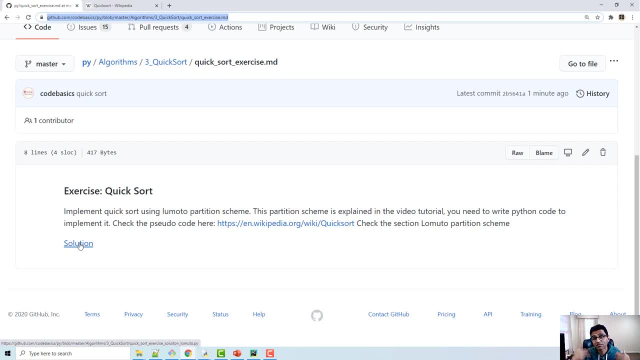 practice, and then only you can learn it by watching my video. you're not going to become an expert. you have to practice, practice, practice, practice practice. I hope you're liking this tutorial series so far. if you do, please give it a thumbs up. share it with your friends on Facebook, whatsapp, whatever medium. I'm 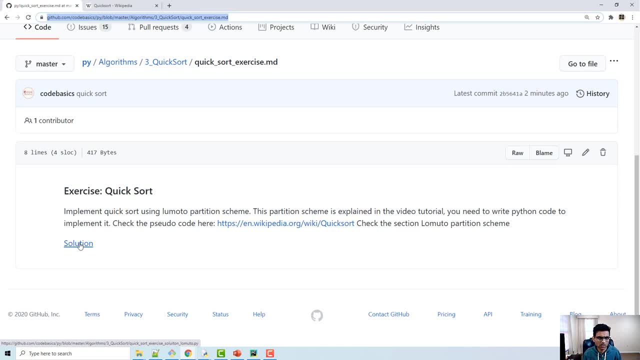 gonna cover many more tutorials actually in this data structure and I'm going to share an algorithm series. I have a link of complete playlist in the video description, so please check it out. follow all these tutorials. data structures and algorithms are extremely important. they're very important during. 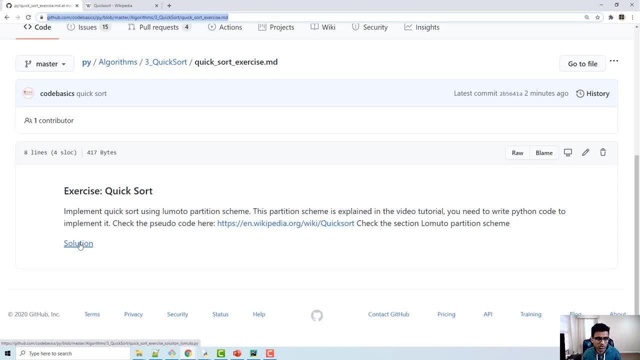 interviews. so if you want to crack coding interview for programmer position, data scientist position, you you have to know this. for data scientist position, I think it's still you need to know not much. but for programmer position, you have to really export into this. alright, thank you very much for watching. goodbye.